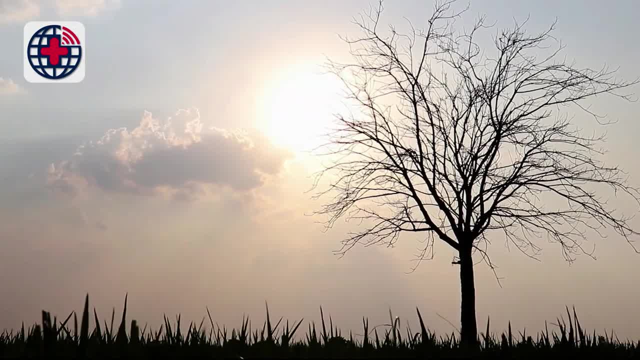 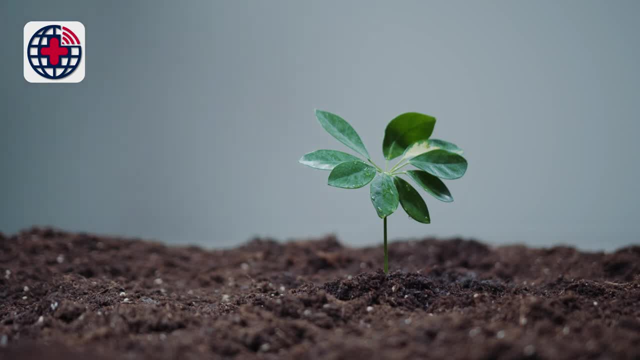 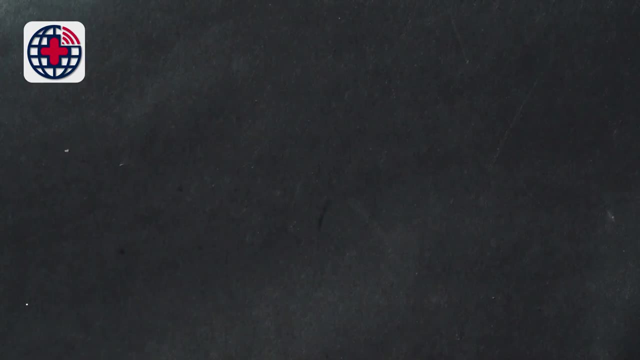 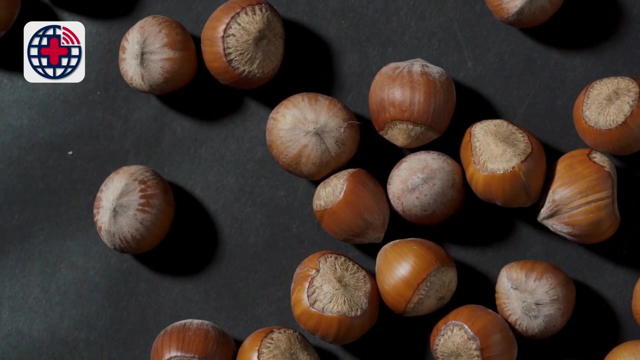 precipitation patterns, increased frequency and severity of extreme weather events and altered growing seasons. These changes can result in decreased food production, reducing food availability and accessibility, and increasing food prices. Food Quality. Climate change can also affect the quality of food, as changes in temperature and precipitation. 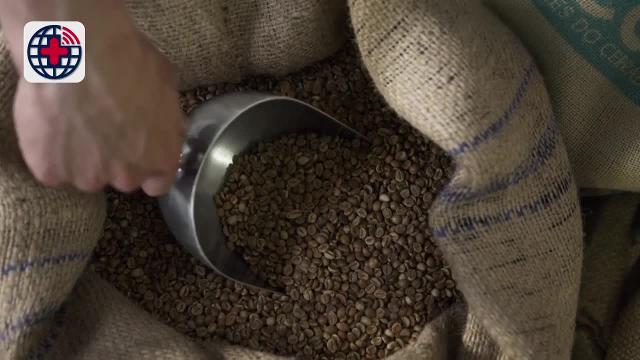 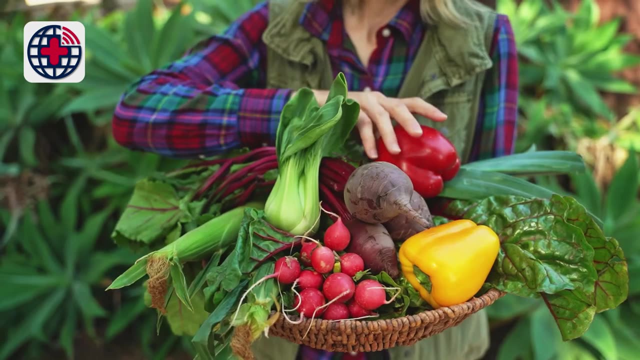 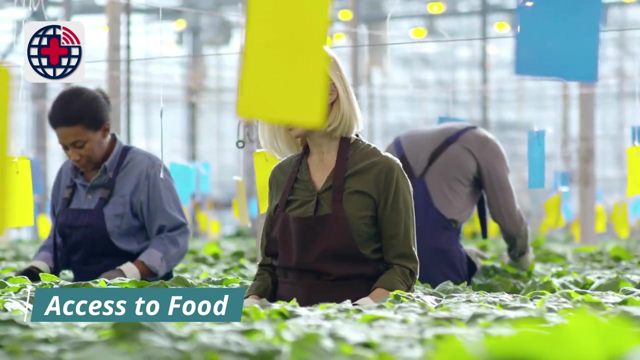 can alter the composition and nutritional value of crops. This can result in decreased food quality, reducing the nutritional value of diets and increasing the risk of micronutrient deficiencies. Access to Food: Climate change can also impact access to food, as changes in temperature and precipitation. 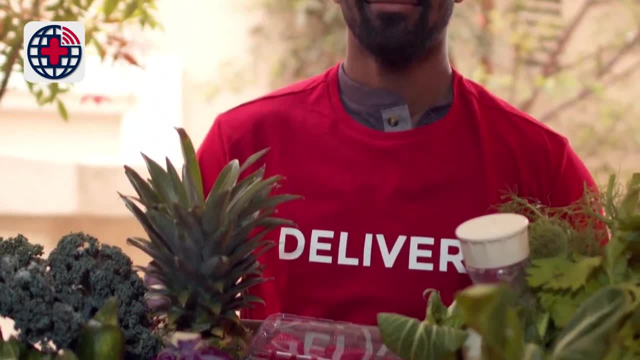 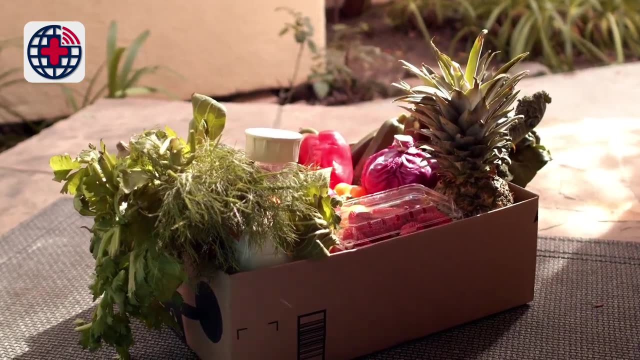 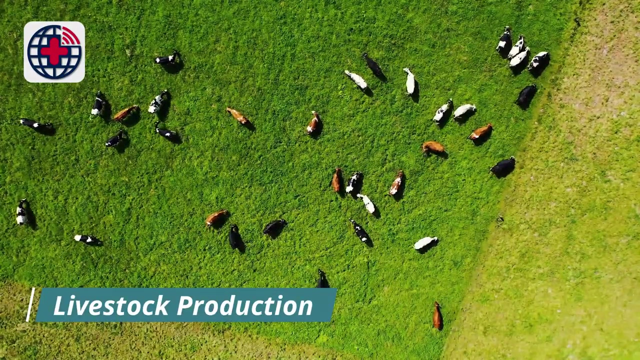 patterns can affect the ability of individuals and communities to grow and harvest crops, and transport and distribute food. This can result in food shortages, reducing food access and increasing food insecurity. Livestock Production. Climate change can also affect livestock production, as changes in temperature and precipitation. 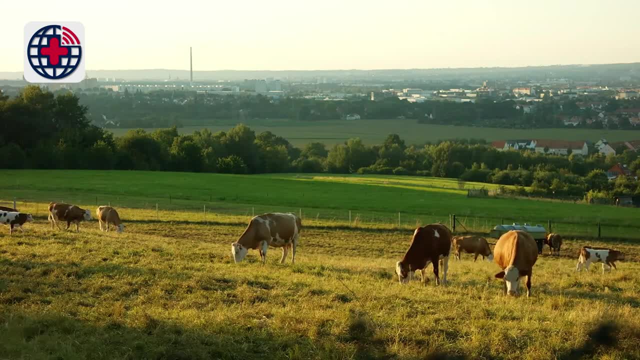 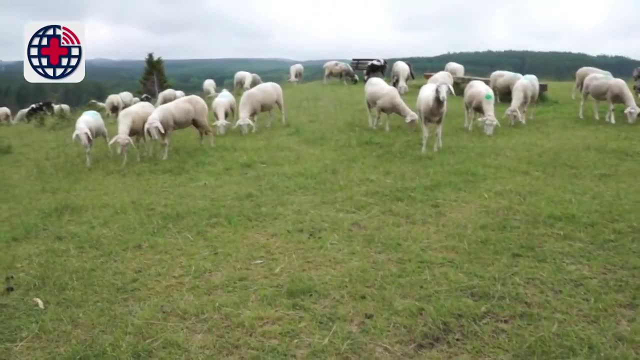 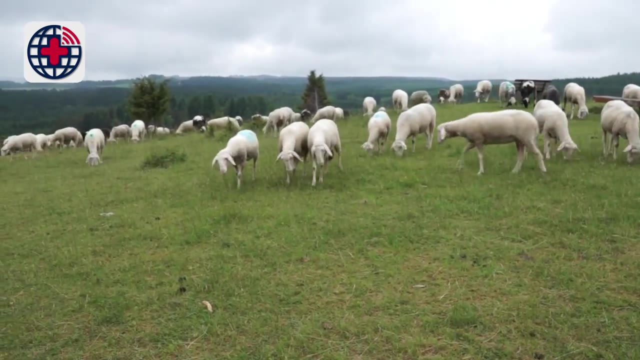 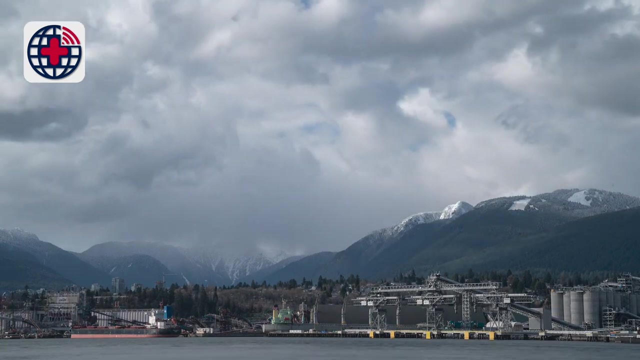 patterns can affect feed availability and quality and increase the risk of diseases and parasites in livestock. This can result in reduced livestock production, reducing the availability of meat and dairy products and increasing food insecurity. In Conclusion, Climate change has the potential to significantly impact food security and nutrition, both directly. 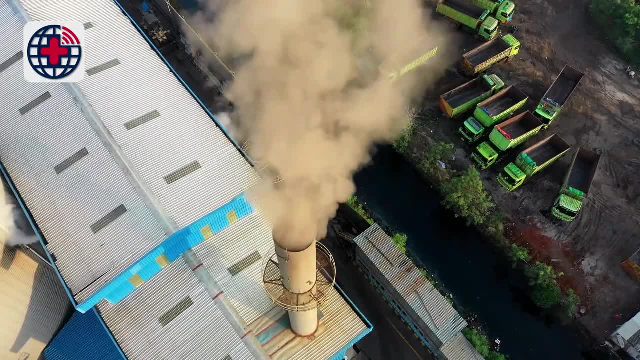 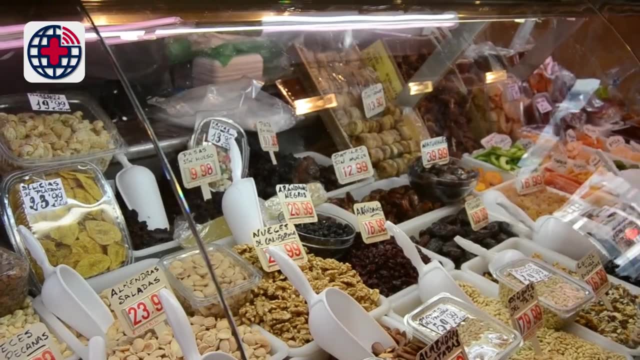 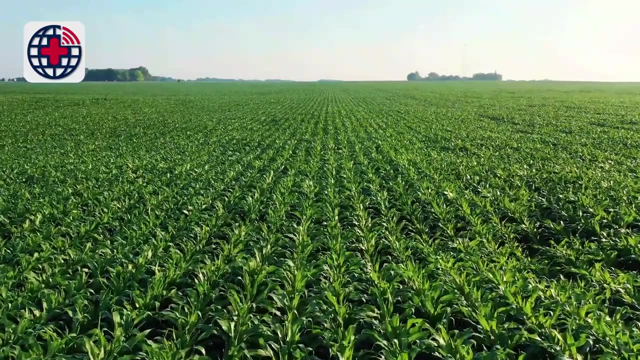 and indirectly, by affecting crop yields, food quality, access to food and livestock production. Addressing the impacts of climate change on food security and nutrition requires multi-sectoral and integrated approaches, including sustainable agriculture and food systems, disaster risk reduction and social protection programs. 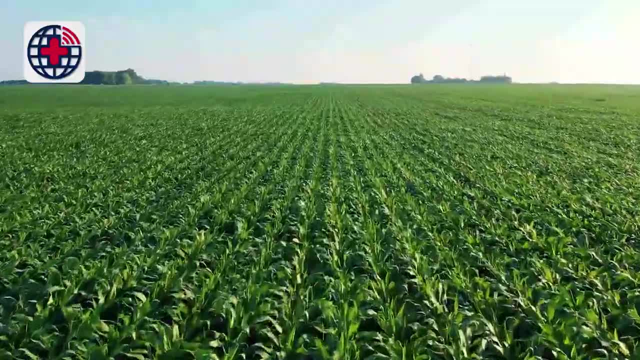 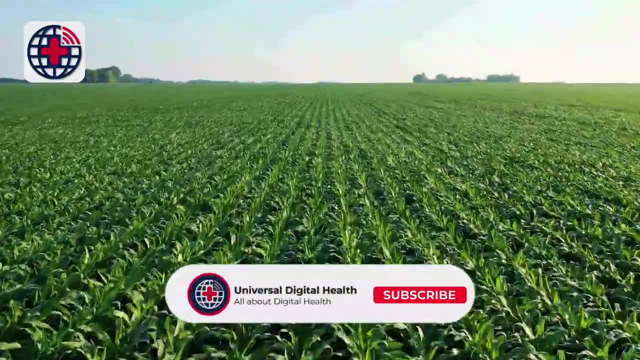 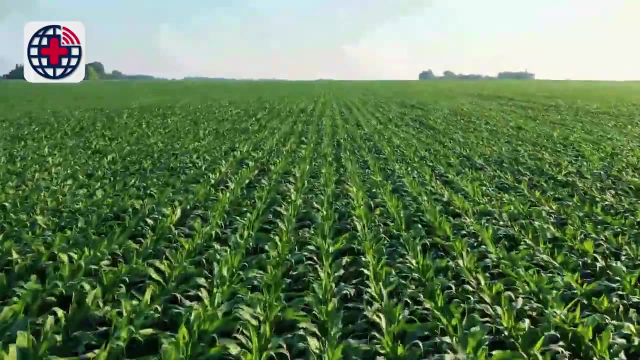 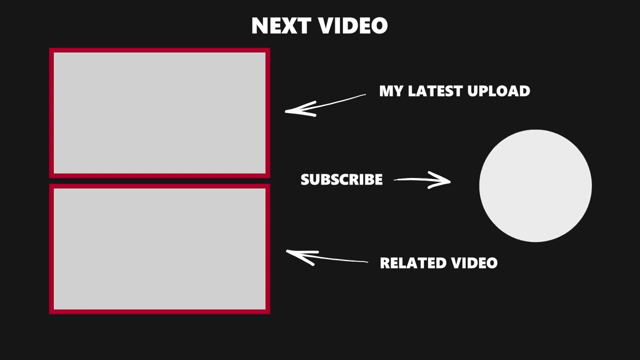 To ensure that individuals and communities have access to adequate, nutritious and sustainable diets. Thanks for watching. If you liked the video, please like the video and subscribe our channel for more digital health content. Thank you.